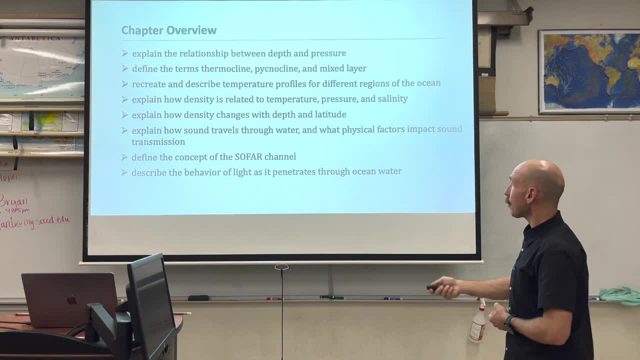 today. So what exactly are we getting into The relationship between depth and pressure, The terms thermocline, pycnocline and mixed layer. We'll look at temperature profiles for different regions and by season and latitude. We'll explain how density is related to temperature, pressure and salinity. We'll explain density changes with depth, latitude, how sound travels through water, what physical factors 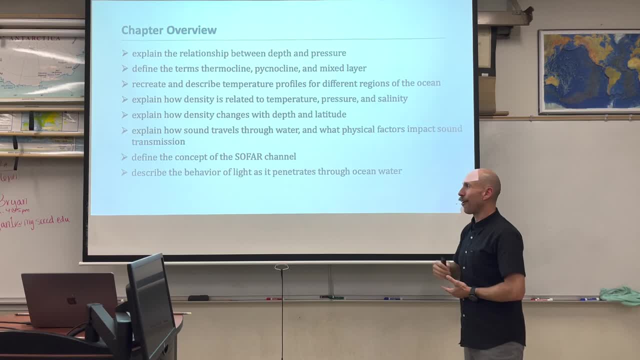 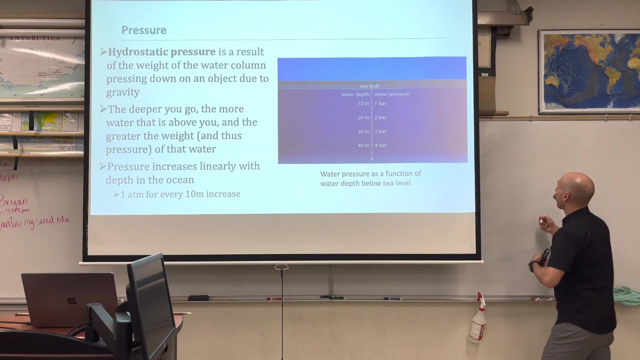 impact sound transmission through the so far channel. It's so far. No, it's actually really cool. Describe the behavior of light as it penetrates through ocean water and round up our discussion on why are oceans blue? Ah, unique characteristics of light. Let's dive right in. So we will begin our discussion of physical 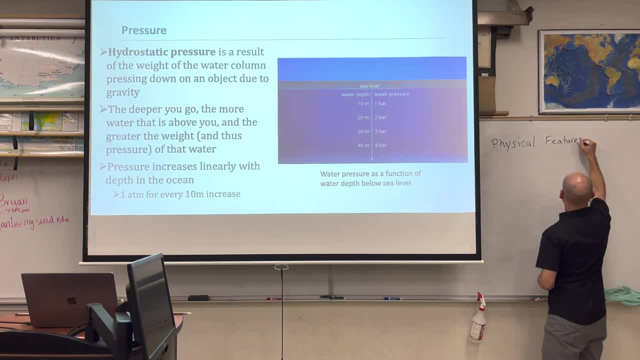 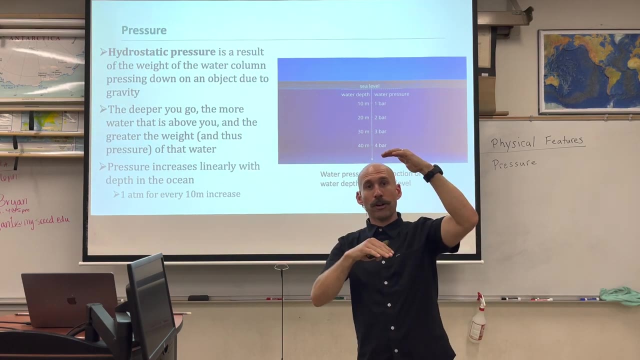 with pressure. Okay, So hydrostatic pressure is going to be the weight of all the pressure of the water column above at a given point. I like to think about this as: imagine you and 30 of your best friends all decide you want to stack up in a 30 person dog pile. 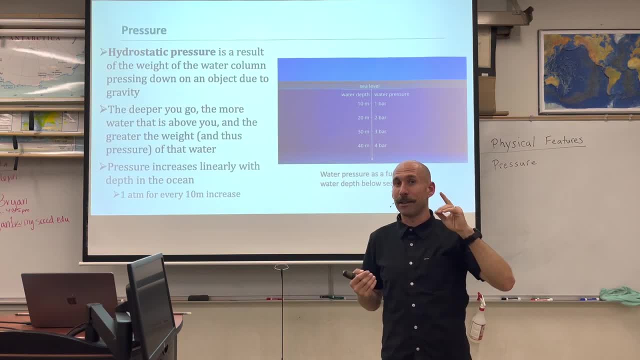 Which person would you want to be? The person on top. Why is that? Because you wouldn't get smashed. It's very intuitive. The person on the bottom? they're going to get smashed Now. think of a water column being those 30 bodies. The 30th body on the bottom feels the overlying weight of all 30 bodies above at the top doesn't feel that, And so this concept of the dog pile is actually hydrostatic pressure. The deeper you go up there, the stronger that pressure will become. All of those three layers of under pressure is going to catch and move. 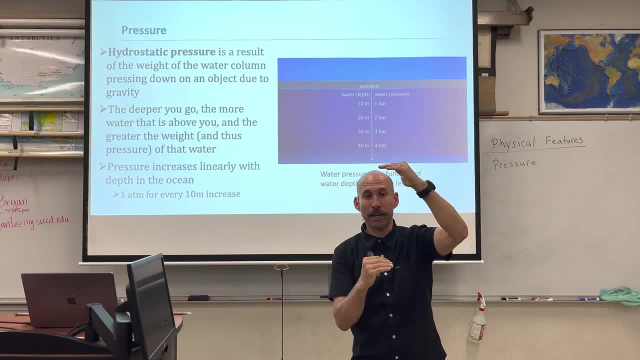 hybrid andincarnationBe. we're going to see a groups of the bastae and intellect And remember we go through столько multiple years in these different environments, these different communities. They were designed, but why do they change at the same time? so people can pay anyway. Now we're going to get out of here one another method that you can enjoy: this way to make. 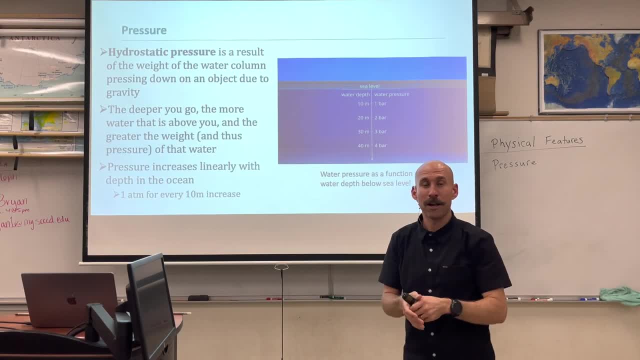 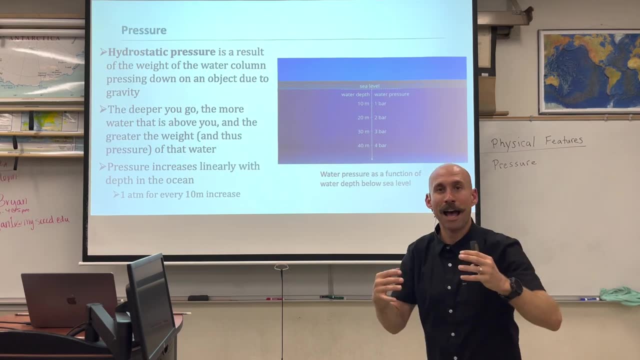 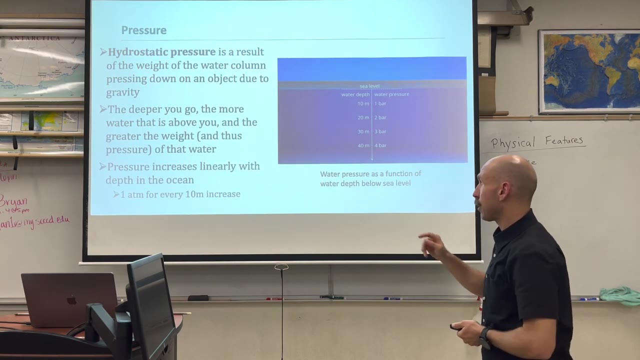 of the dog pile is actually hydrostatic pressure. The deeper you go in the water column, the more you feel the weight of the overlying water above that point. So pressure increases with depth in the oceans. And how much does it increase? Well, on the surface, atmospheric pressure is: one ATM. Every 10 meters increase in ocean depth, we have an increase of one ATM. So sea level one ATM 10 meters down is going to be two ATMs, or one bar 20 meters down is going to be three. 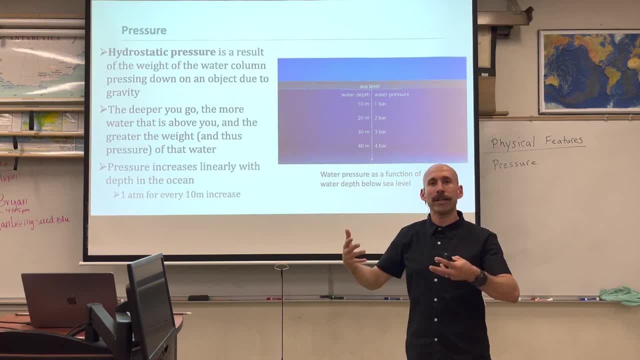 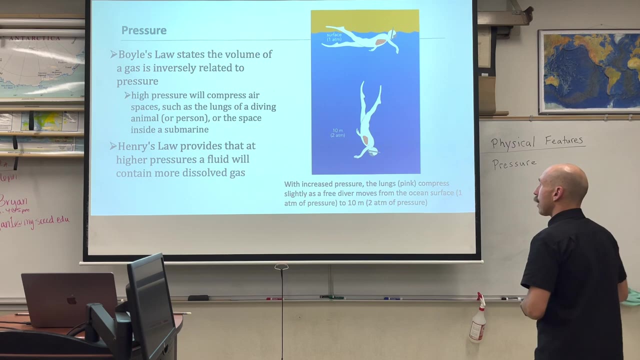 ATMs, or two bar, so on and so forth all the way down. Bars are another way of measuring pressure, So deeper you go. it is a linear relationship of depth and pressure. one ATM for every 10 meters. Now, when you have 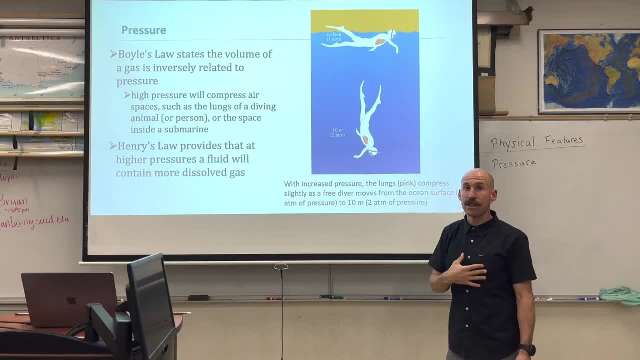 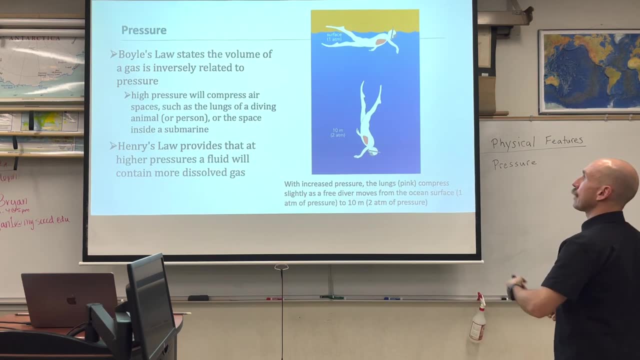 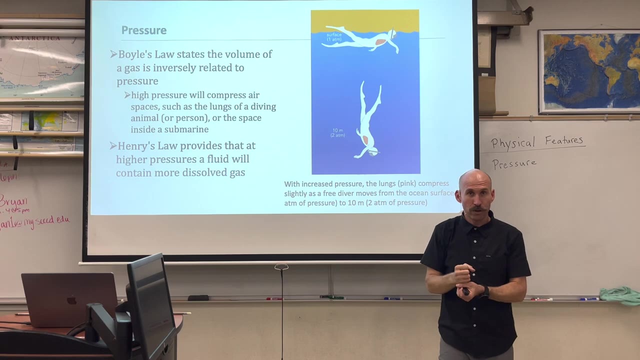 collapsible spheres like the human lung, interesting things will happen. According to Boyle's law, the volume of gas is inversely related to pressure, So that means as the pressure goes up, the volume goes down. This causes this happens inside of lungs of humans. it also happens inside of whales. Whales are some of the deepest divers. 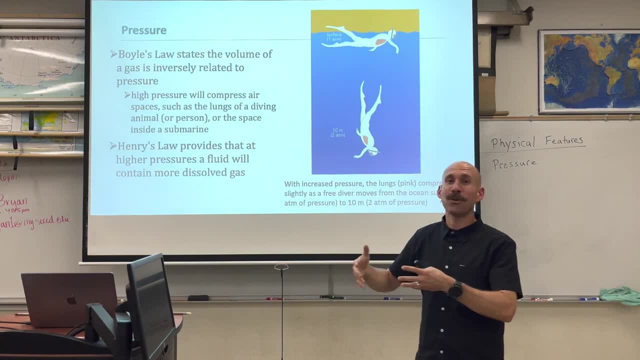 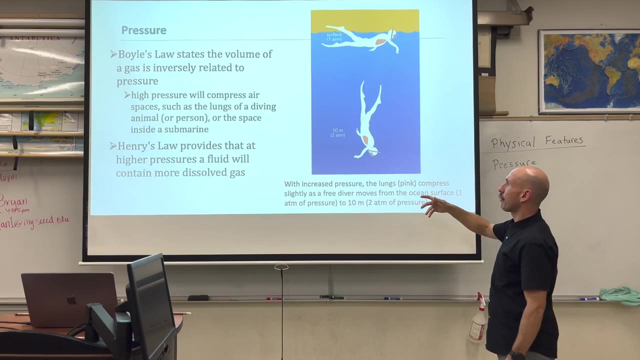 in the ocean, of which our discussion when we get to marine vertebrates is going to blow our minds. it will be awesome, But for now we can say that gas is compressible. where liquids are not so compressible, Henry's law provides that at higher pressures a fluid will contain more dissolved gas. 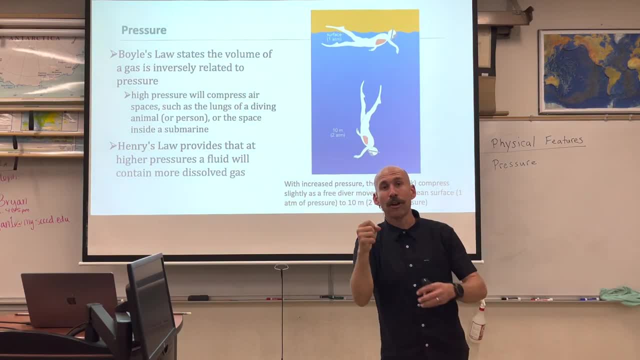 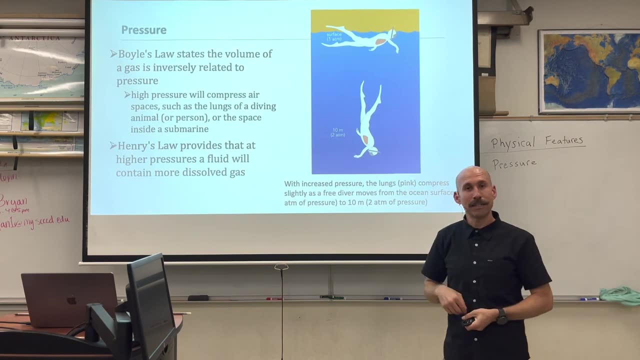 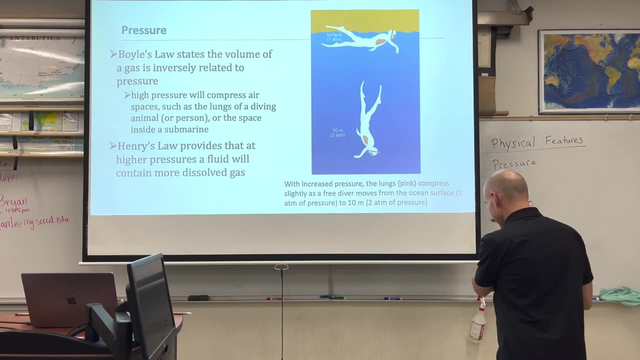 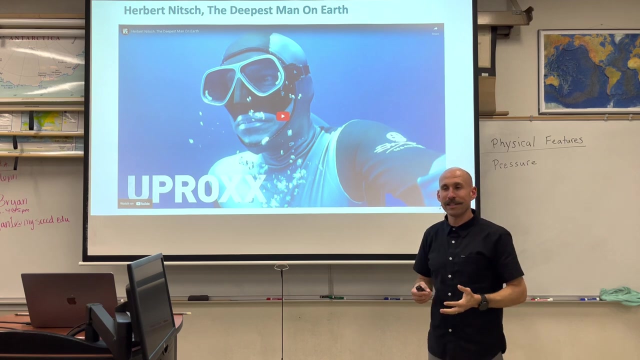 because those gases compress and are able to be contained within the liquid which they are traveling. So lots of dissolved gases down deep in the bottom of the ocean where the pressure is immense. Excuse me, Please view my deepest man on earth. This is more fun than science, but also science, because science is fun. So check this out. 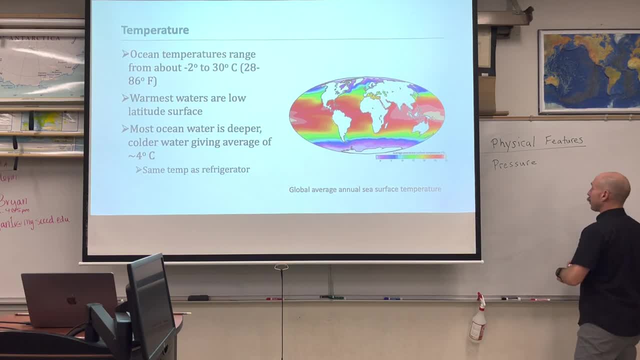 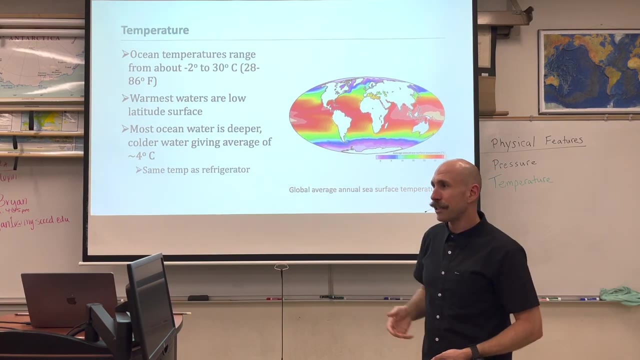 All right, Pressure: Here is our next physical feature. Next, pressure increases with depth. Temperature: Here is our next physical feature. Temperature is kind of cool. It ranges from about minus two degrees of 30 degrees celsius. 30 degrees celsius is pretty warm, but the average temperature. 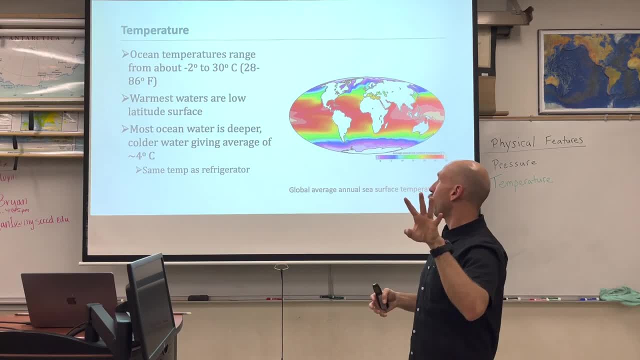 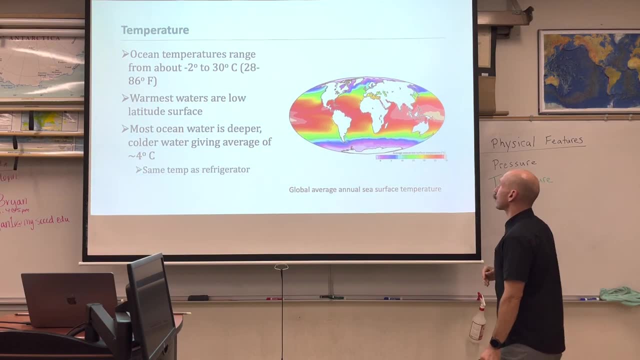 if you take all the temperatures of all the oceans is about four degrees celsius. This is the same temperature, roughly your refrigerator. the sea surface temperature here we can see in equatorial temperate regions gets up to 25, even 30 at the poles. it's a little. 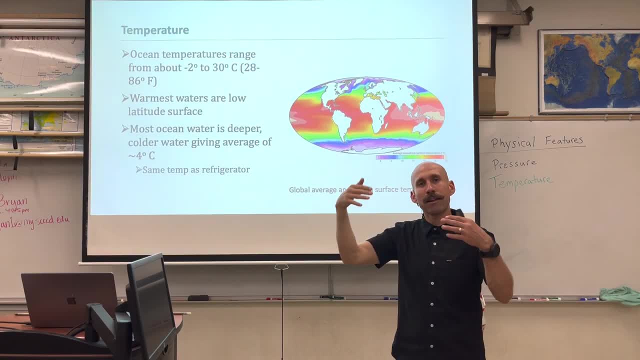 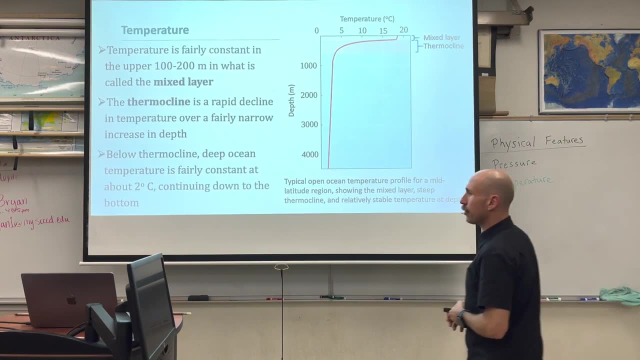 bit lower: 0 to 5. that's just the surface. but let's get a little bit deeper. let's see what's underneath of the surface, shall we? according to our graph, we can see that temperature on the surface is higher than underneath of the surface and in fact, this upper part, the upper 100 to 200 meters, is called the mixed. 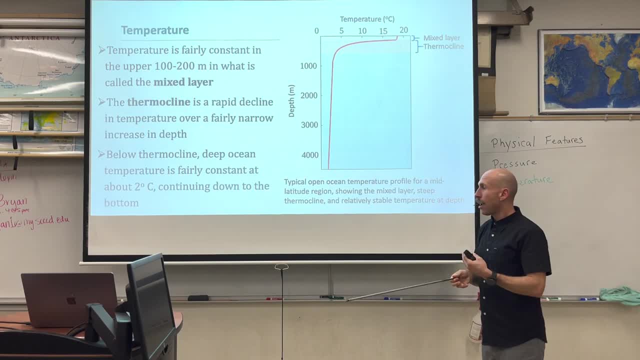 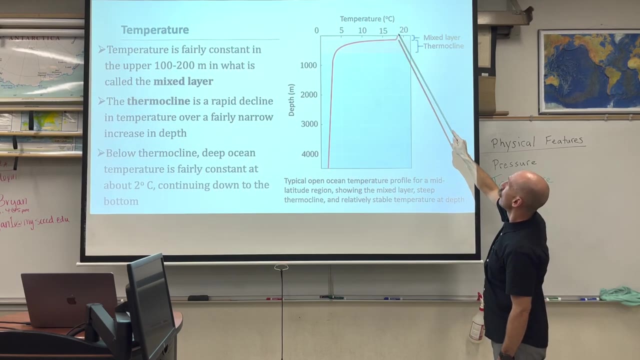 layer where you have a lot of wave action, marine life action. lots of things are happening up here in the mixed layer. underneath that, you have a rapid decline in temperature in what is called the thermocline. so the thermocline exists from about 200 to 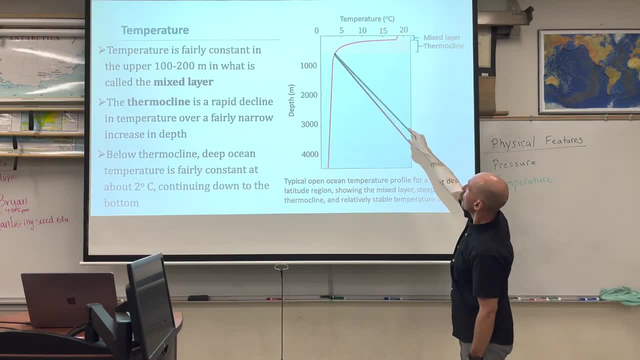 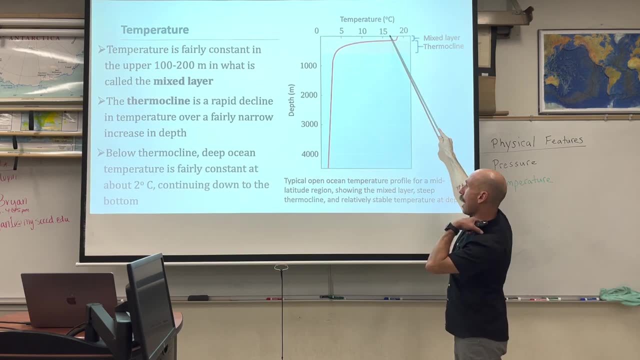 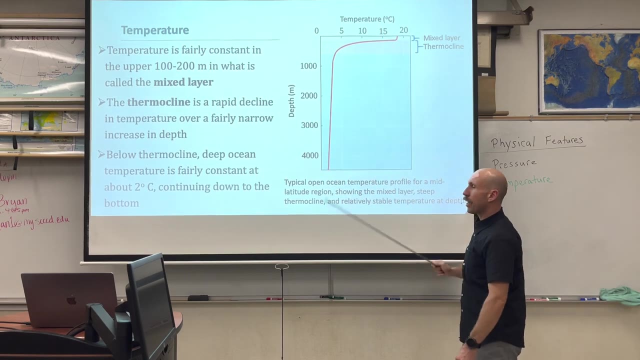 500 meters underneath the surface and below the thermocline temperature levels. out here we have depth on the y-axis, temperature on the x-axis, and it evens, it stabilizes to about 2 degrees all the way down to the bottom of the ocean floor. so this is pretty cool. 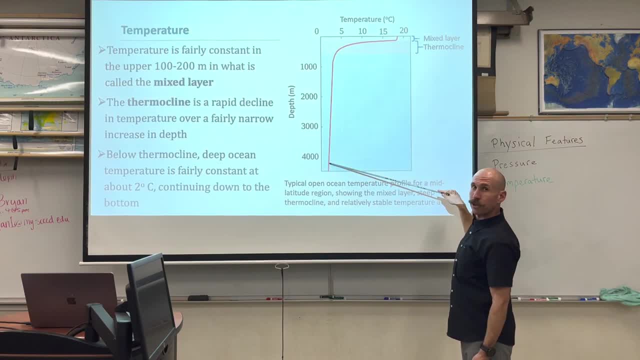 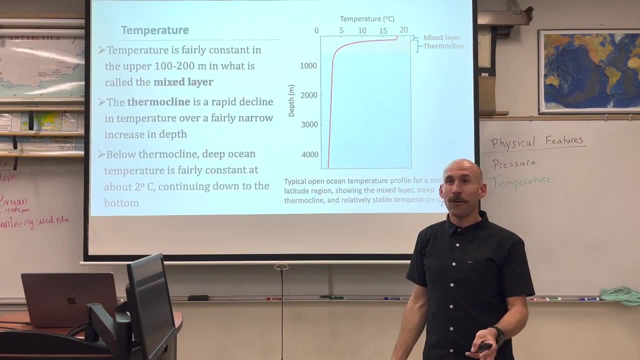 warm at the surface surface, real cold underneath the surface And if you've ever been swimming at the beach you notice it's not freezing. There's some oceans that are really cold. The Pacific is much colder than the Atlantic. That has to do with subtropical gyres and atmospheric circulation patterns, because the 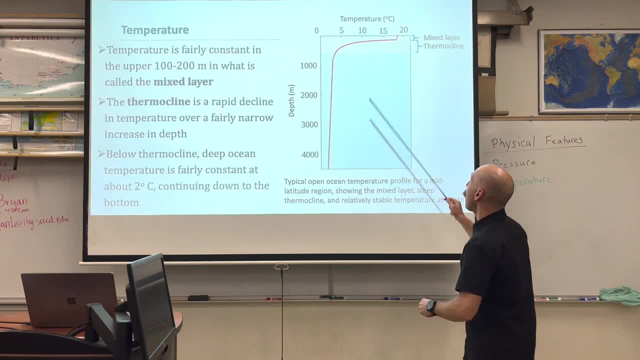 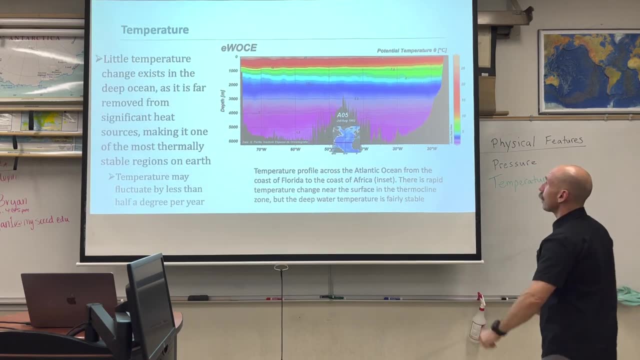 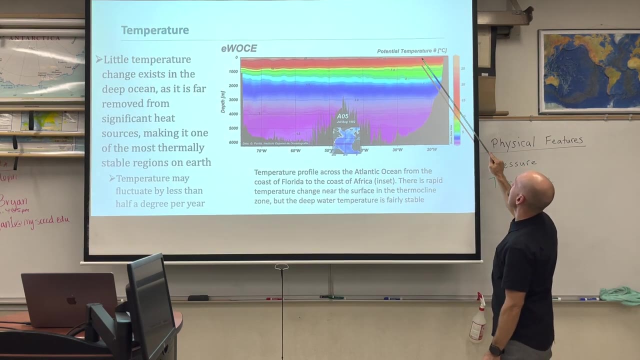 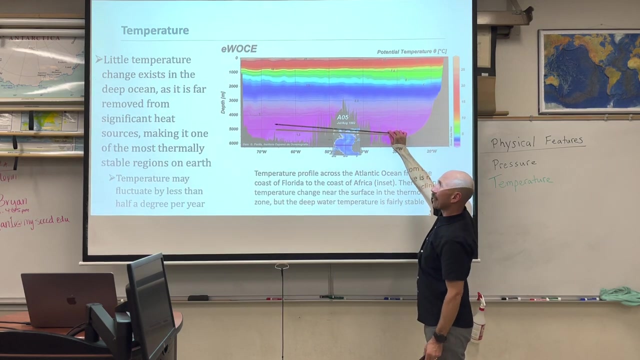 earth spins on an axis. It's really awesome. We'll talk about all that- But warm at the surface, stable and cool in the subsurface. So if we look at the entire ocean floor, what we see here is that the potential temperature change is much higher at the surface and really low, In fact, the bottom. 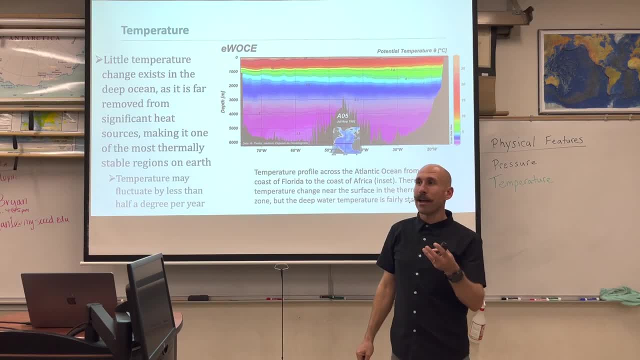 of the ocean is one of the most stable areas for having a temperature that doesn't change. It fluctuates by almost a quarter of a second. So if we look at the bottom of the ocean, it's one of the most stable areas for having a temperature that doesn't change. It fluctuates by almost a 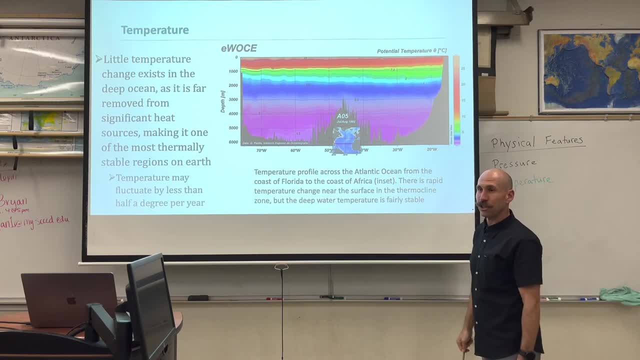 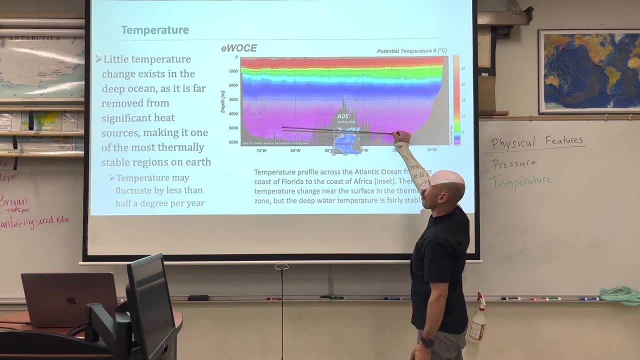 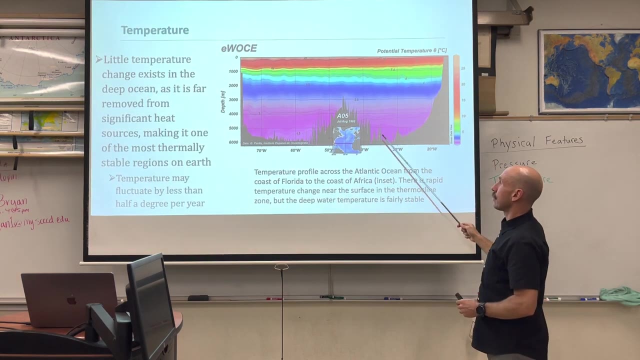 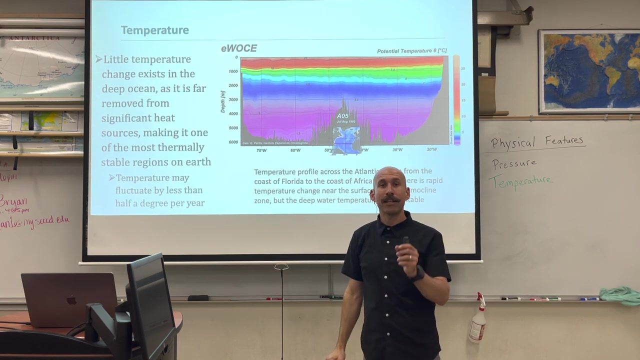 degree down here, which allows for stillness. It allows for the water to sit down here for long periods of time. About how long? Oh, we'll have to wait until ocean circulation. But the fact that there is a temperature gradient as defined by warmer at the top, cooler at the bottom, has a huge 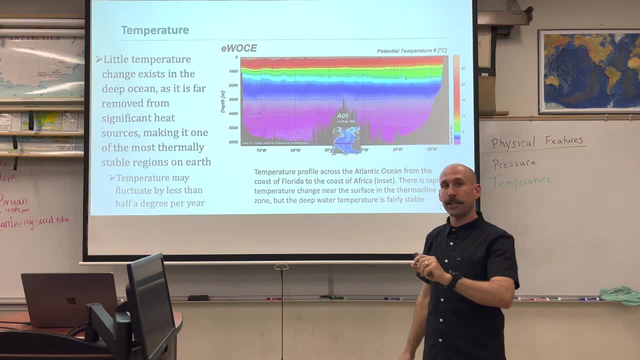 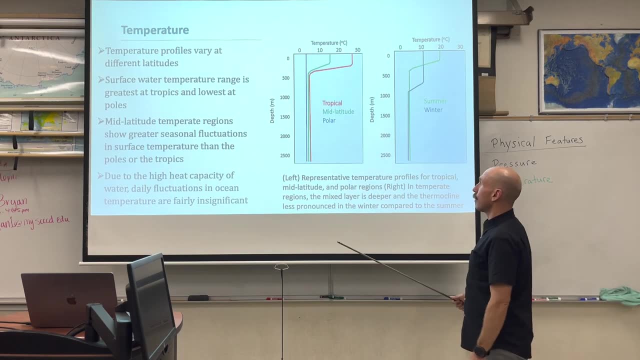 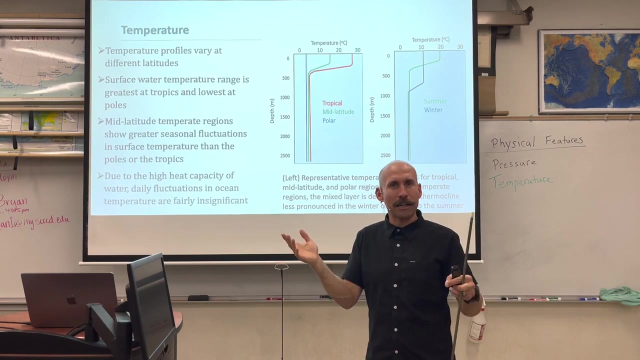 influence on global oceanic circulation patterns. So if we think about temperature, it varies by latitude and by season in temperate regions. So we can think about an equator. It's like hey board shorts swimming in the ocean, It's hot. The poles, Antarctica, it's cold. So you would expect in cold places, cold surface water And in warm places warm surface water. 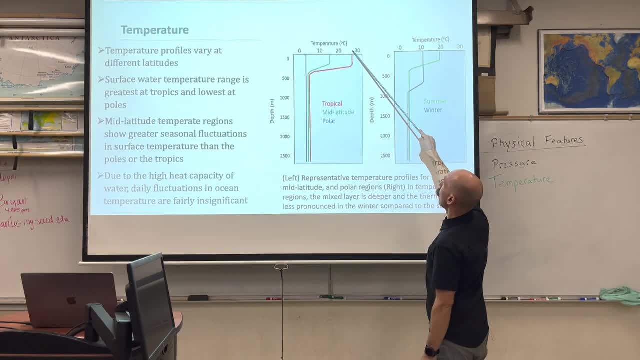 That's what we see. Red line: tropical warm surface- Here's the thermocline And then at depth about the same temperature as mid-latitude and polar Mid-latitude doesn't get so warm Thermocline. for polar regions the thermocline is absent. 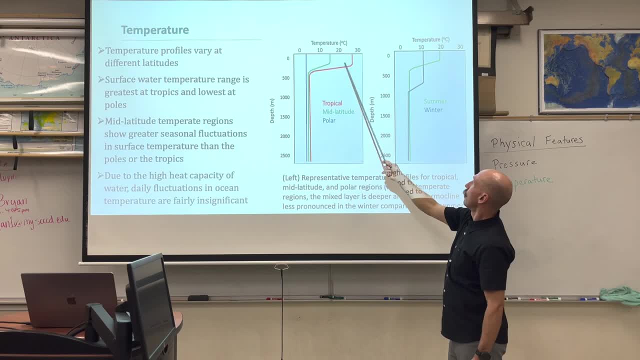 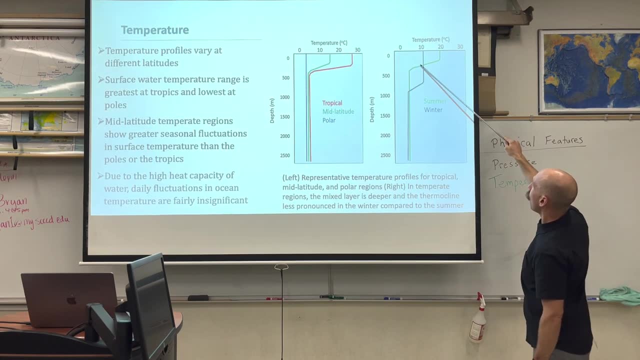 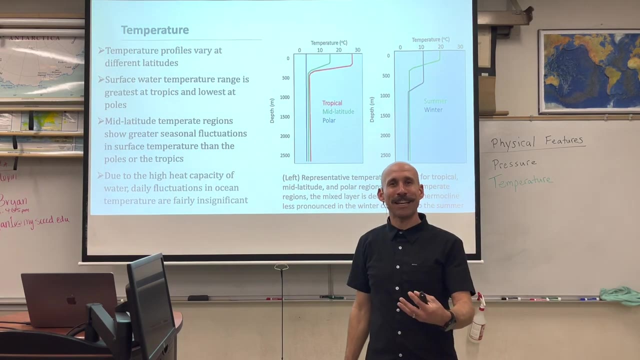 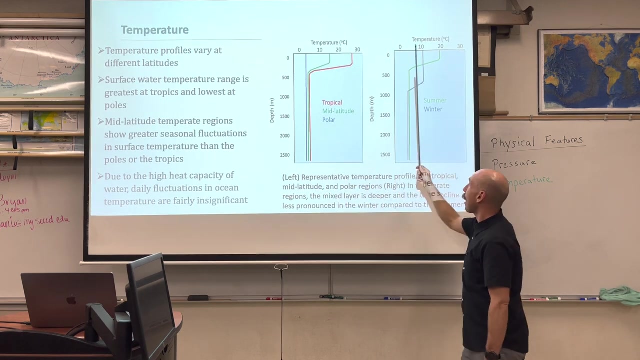 Now let's take these tropical, mid-latitude temperate climates. The thermocline actually shifts up and down In the water column from summer to winter, depending on how much solar radiation is available to warm up the environment. So the big two by latitude and by season in temperate climates is going to affect the temperature regime and where the thermocline is. 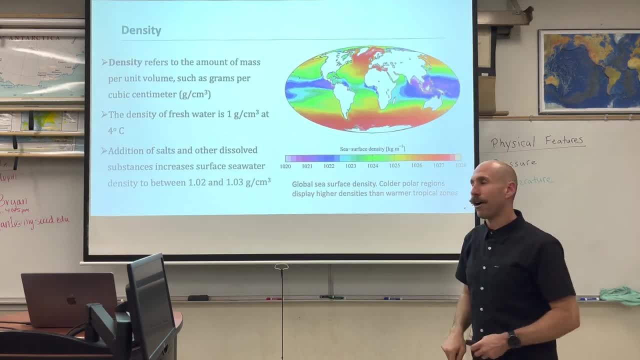 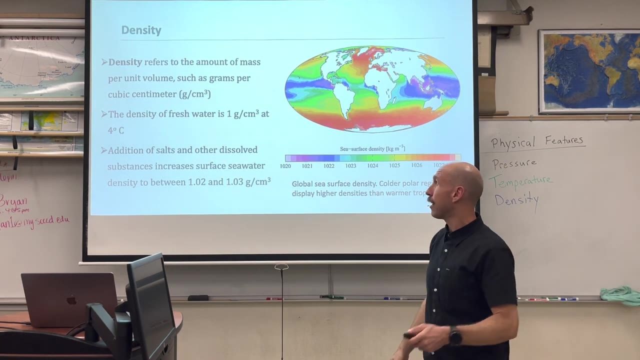 Very good. Continuing on Dense: Whoa, that's dense About how dense? Well, at the average temperature of ocean waters, 4 degrees Celsius, about 1 gram per cubic centimeter. So this is a mass. per volume, Gram is a mass. 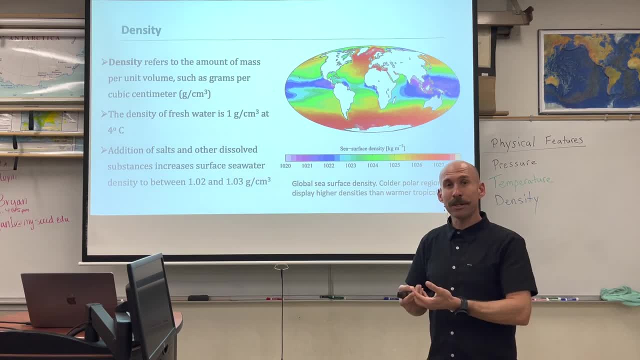 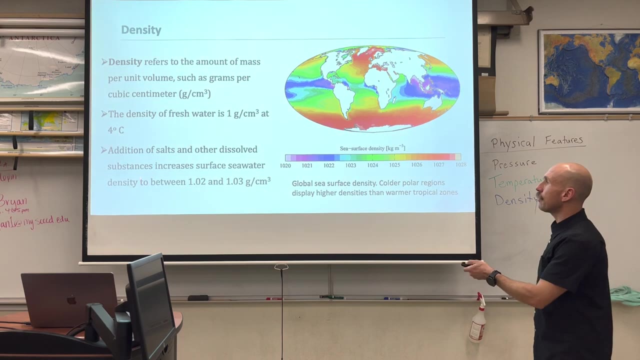 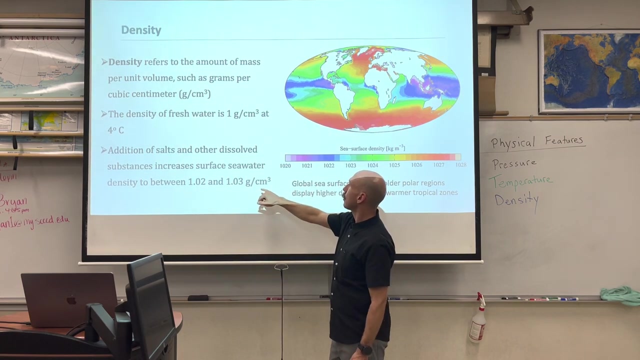 And cubic centimeters is a volume. Now density can shift based on temperature, based on the addition of dissolved substances increasing its salinity, And so we get seawater density that on the surface that can vary between 1.02 and 1.03 grams per cubic centimeter. 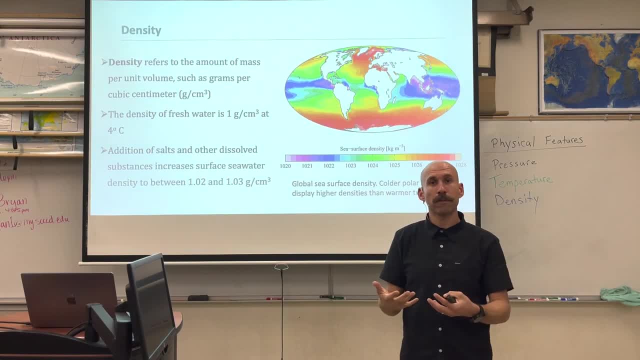 So we have these averages. So we have these averages, which are good for understanding, but the world is complex and the oceans are complex, just like you and I are both complex, and there are nuances and there is variability and there is all these interesting things happening. 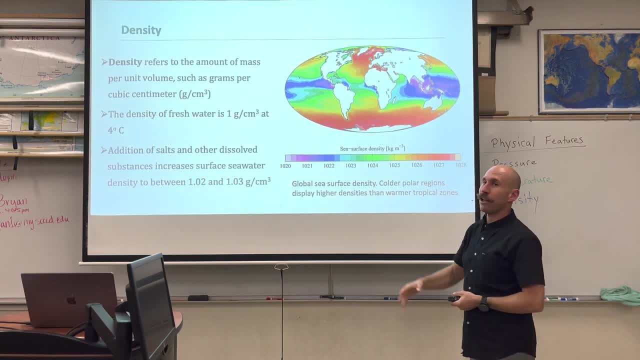 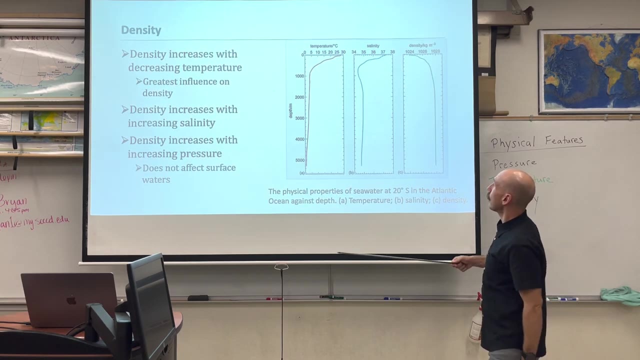 and there is variability and there is all these interesting things happening. It's good to understand on a global scale, but we also need to take into consideration more granularity to understand how these systems function as a whole. So, if we think about density, here we have a graph of temperature, mixed layer, thermocline. 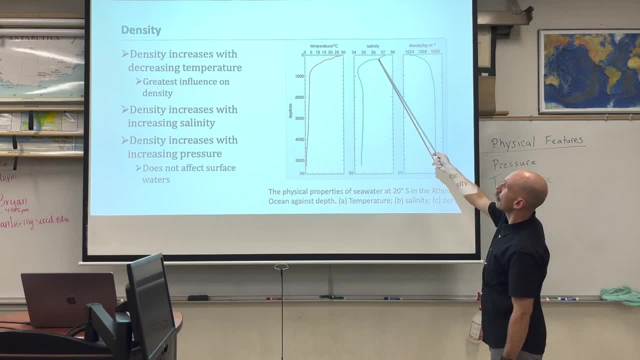 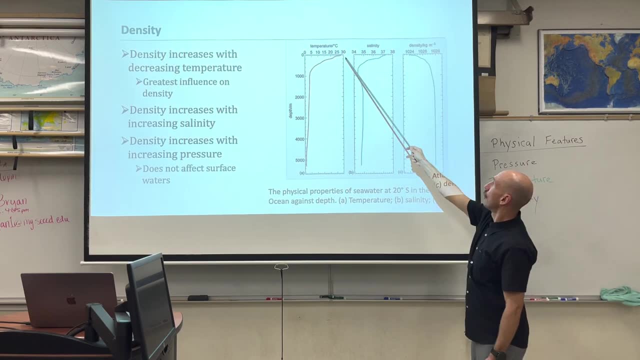 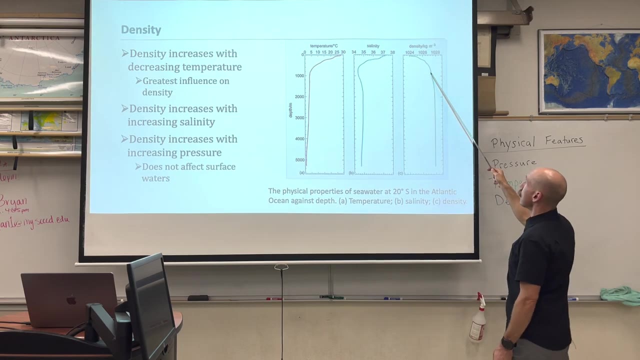 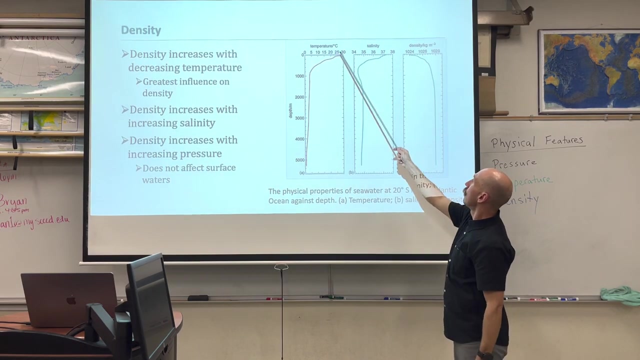 deep ocean salinity and density. We have something very similar happening. Notice rapid change in temperature. rapid change in salinity, that's called the halocline. rapid change in density, this is called the pycnocline, Where what we really want to take home from this is surface on the y-axis. From the surface. temperature decreases at depth, salinity decreases at depth. density increases at depth and this makes sense because density has to do with pressure and pressure is related to depth, So the density and the pressure are going to increase with depth. 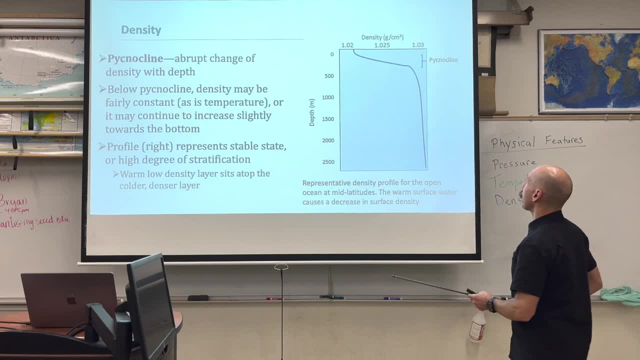 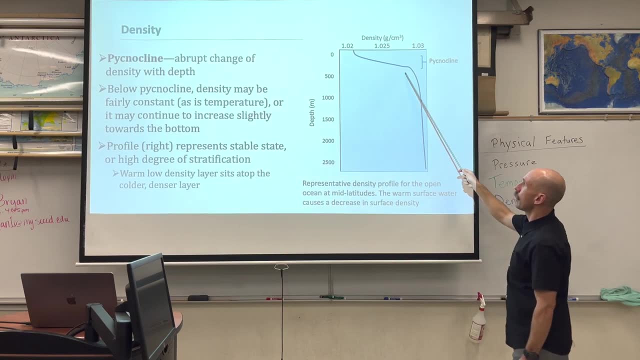 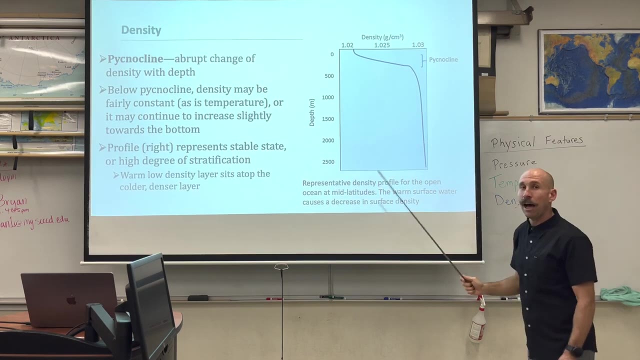 Okay, cool stuff about density. I know Here we go if we zoom into density. pycnocline, an abrupt change in density with depth Below the pycnocline. density is fairly constant because temperature is constant and salinity is constant. 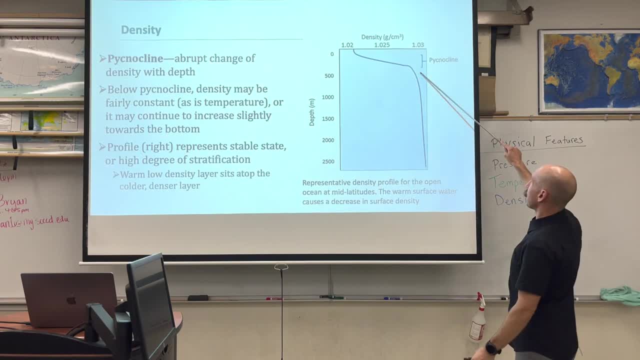 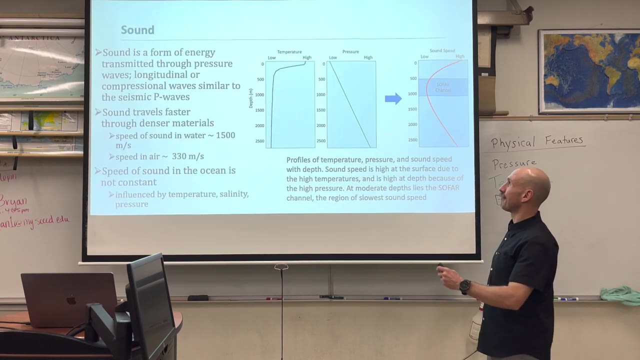 That is awesome. So here we have a stable state with a high level of stratification where we have a warm low density layer sitting on top of a colder, higher density layer. Great things are happening in the ocean Sound. Let's continue on with our next physical feature of the ocean. 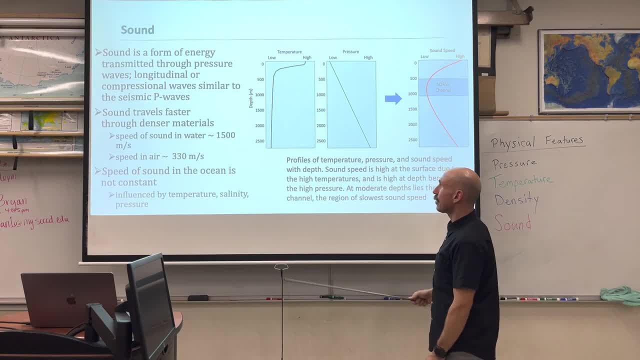 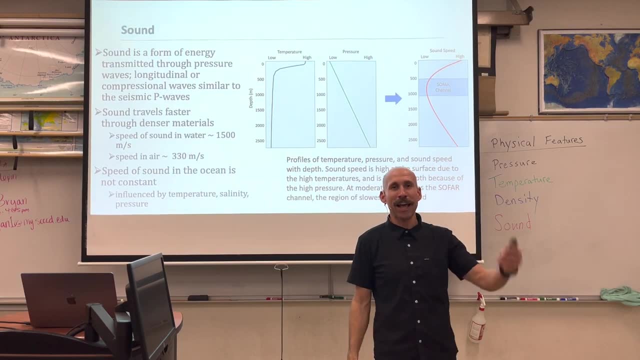 Sound. Okay. so sound in water goes about 1500 meters per second and in air it's about 330 meters per second. What the heck? When I talk underwater, I can't hear anything. Well, that doesn't mean that sound isn't traveling, actually. Sound through water travels very fast. Sound through water travels very fast. Sound through water travels very, very fast, Almost five times faster. And not only that, but the speed of sound in the oceans is not constant. It's influenced by temperature and pressure and salinity. 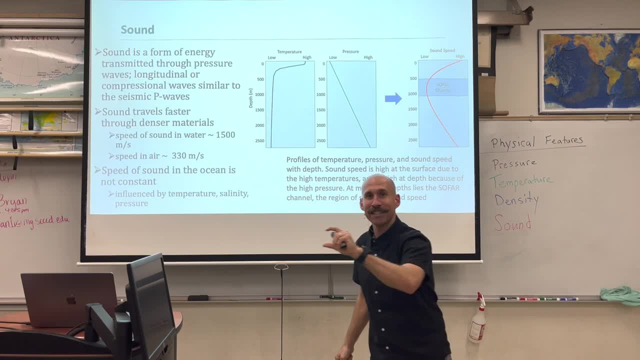 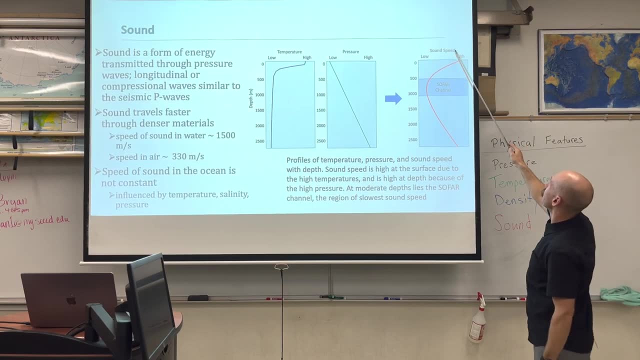 and there is actually a tiny band in the ocean from about 500 to 1000 meters called the SOFAR channel, where the speed of sound is the lowest, but it bounces up and down And it goes back and forth up and down through this cavity. 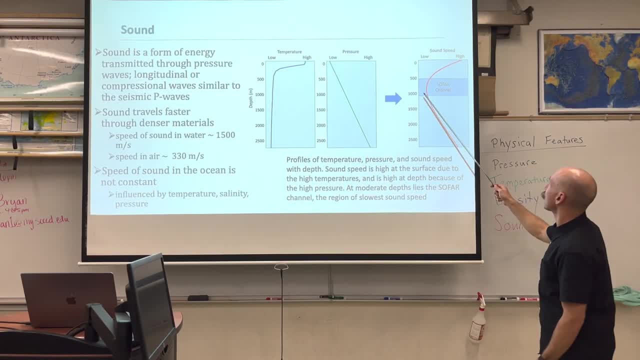 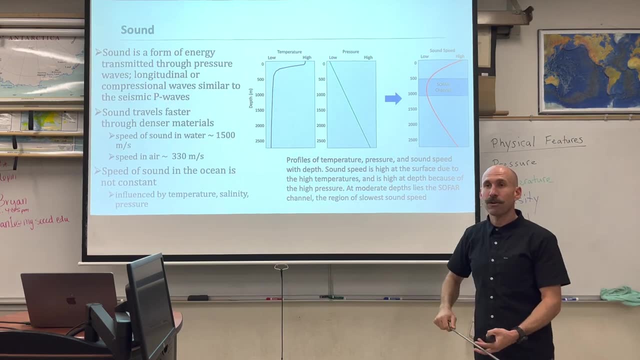 in a way that's similar to seismic pressure waves. So this is really important for understanding how sound moves and also for picking up sounds that we hear in the ocean, Sounds from marine life, sounds from vessels such as submarines or naval ships. The SOFAR is 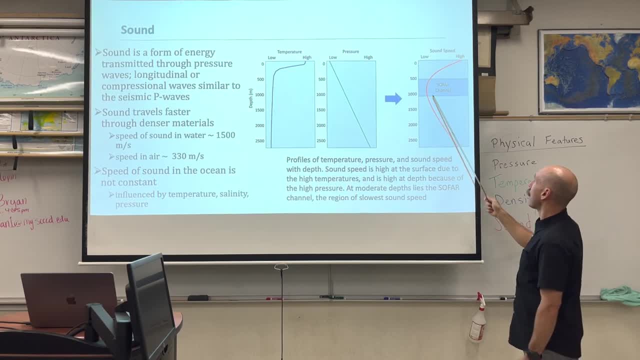 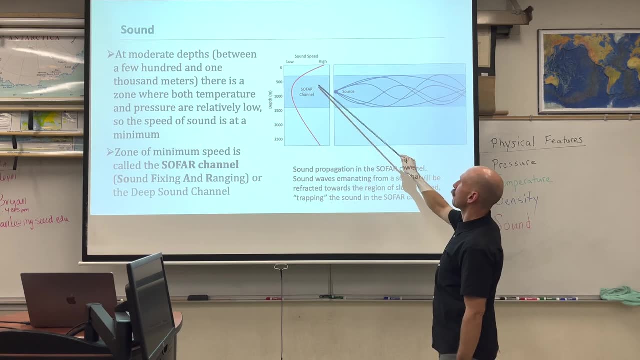 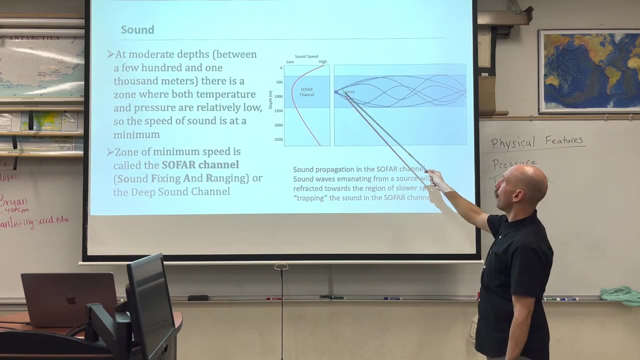 a very important for us to understand, for understanding how sound works in our oceans. So here we go, The SOFAR channel, at moderate depths, roughly 500 to 1,000.. This is where temperature and pressure are both relatively low. 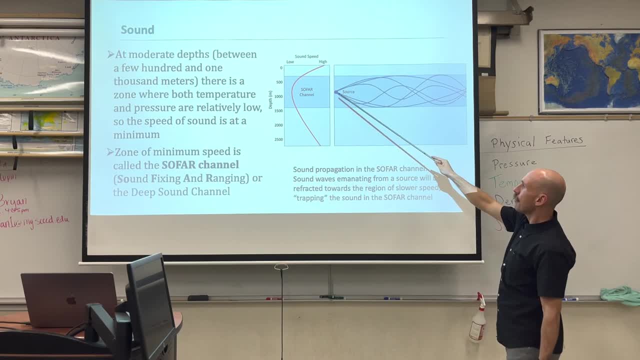 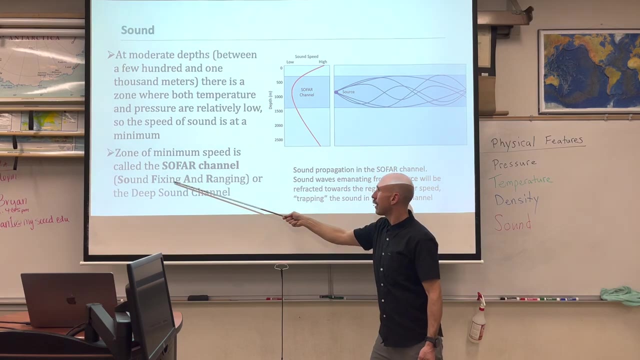 So the sound is at a minimum, but the sound in here is able to bounce off of the top and the bottom this banding of cooler, less dense or, I'm sorry, warmer less dense, cooler, more dense in this channel called the sound fixing and ranging. 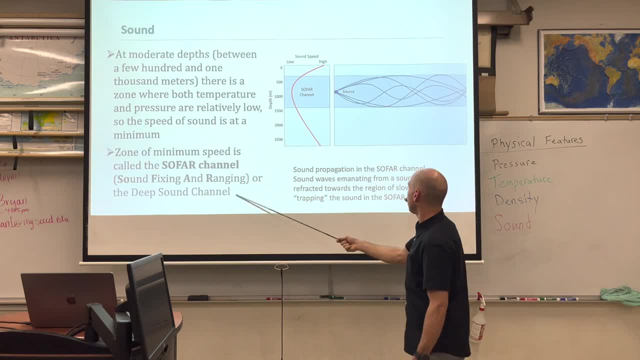 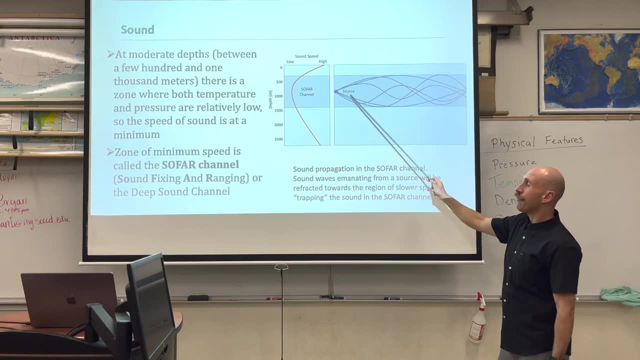 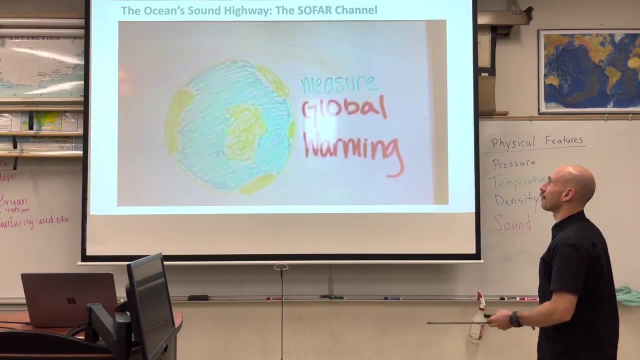 or another word for this, is the deep sound channel. Essentially, the sounds are bouncing back and forth and they're trapped and they can travel extremely long distances within the deep sound channel. Check it out More on the SOFAR channel in the show notes. 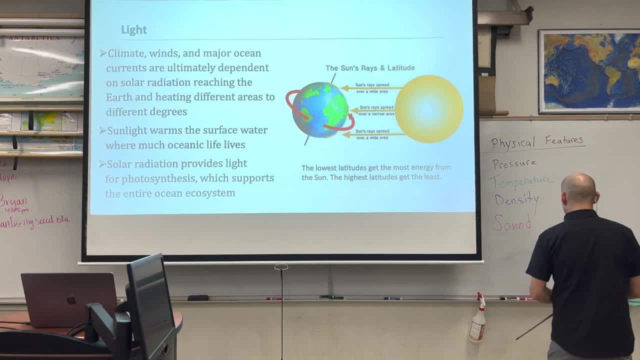 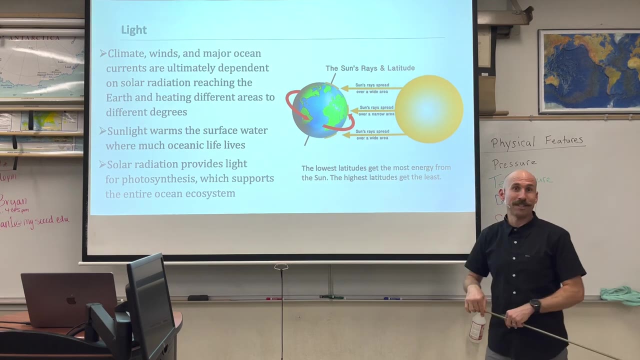 It's available in the description. Check out the videos. We got it Okay. Last but not least, let's talk about light. Light's pretty cool. Comes from the sun, helps us see. It does a whole lot more than that. 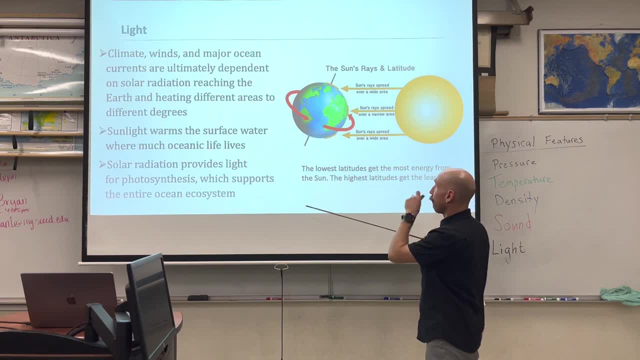 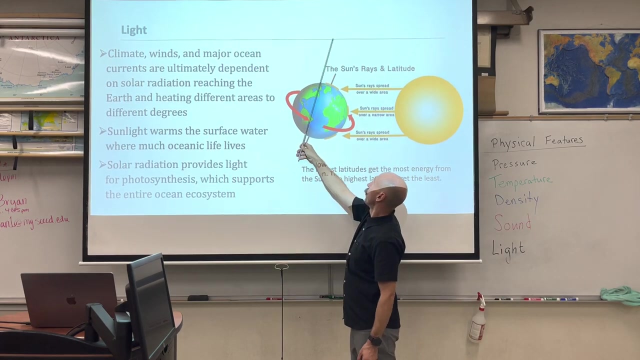 So light is responsible for climate, winds, major ocean currents, and it's more than just light. It's the heat transfer from the sun- solar radiation represented by the electromagnetic spectrum- And it's diverse in how it arrives to earth, because earth is on a 23 and a half degree axis. 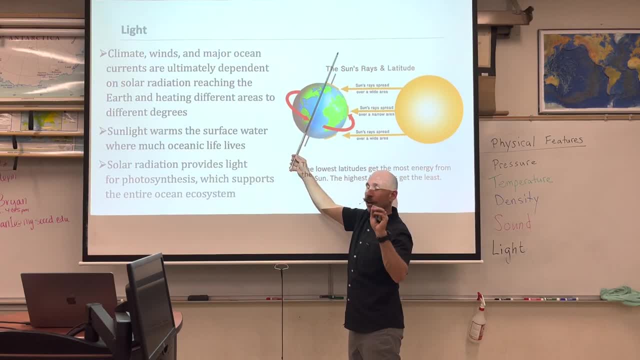 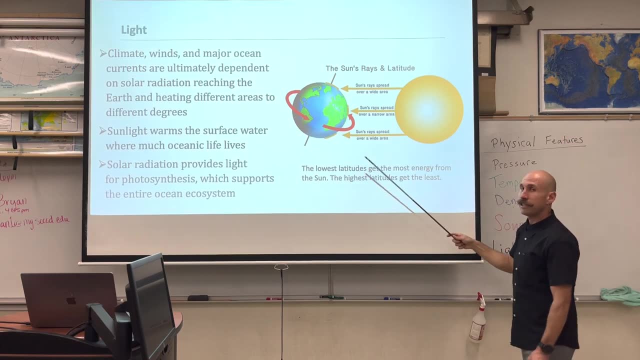 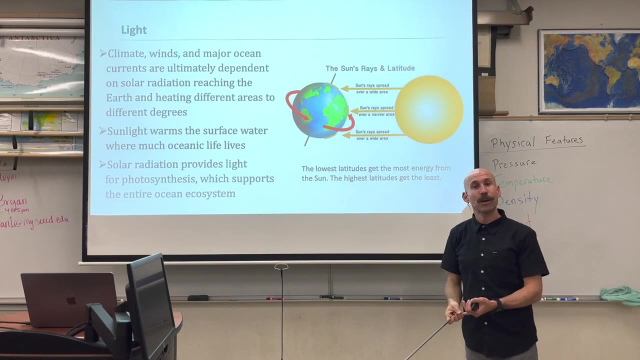 that always points towards the north star, Currently, at this point- not forever, but right now in our human lifetime- and it rotates on that axis. there is a differential heating of the poles and the equator. This gives us seasons and equinox and solstice. It causes also because the earth orbits around the sun Once every 365 years. we get lots of light in the north, in the north pole, and lots of dark in the north pole. that switch every year. Same thing with the south pole. The solar radiation is great. 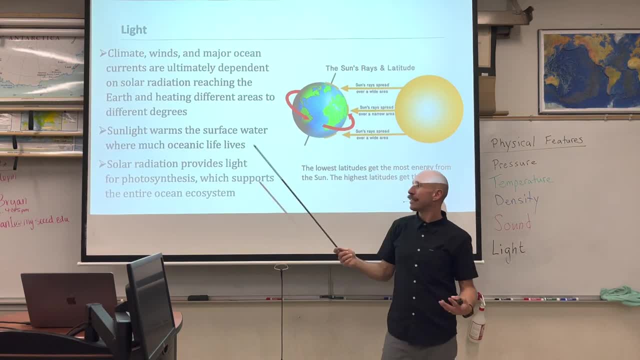 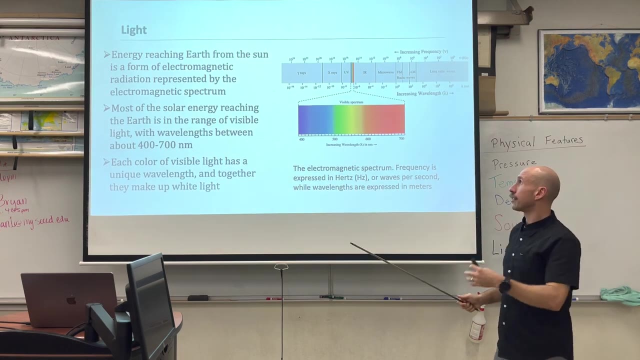 It provides light for photosynthesis which supports the entire ocean ecosystem. So thank you, sun, for supporting everything in the ocean. It's amazing, Even though it's reach is limited for reasons which we'll get into here soon. So energy from the sun, solar radiation, it's heat. 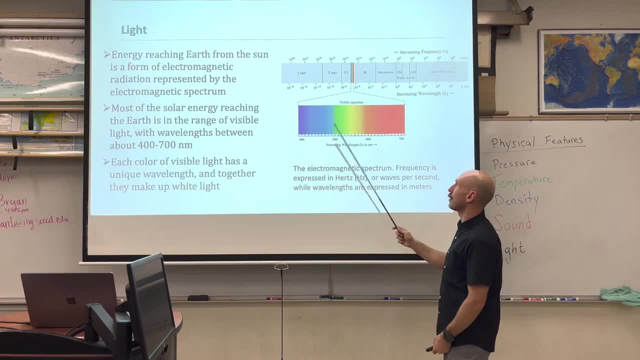 Heat is a form of energy. It's a we record. the energy of a substance, of a material arrives in the electromagnetic spectrum, Which are wave lengths of the light that is arriving. Visible light is a very small portion of this, within about 400 to 700 nanometers. 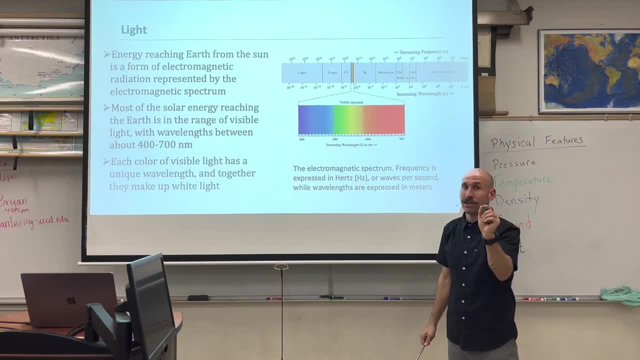 which are very, very small. It's short wavelength that's arriving, So sure we can't see it, And our eyes are really amazing at interpreting what we have going on and allowing us to see color, Because different objects in the world absorb light. 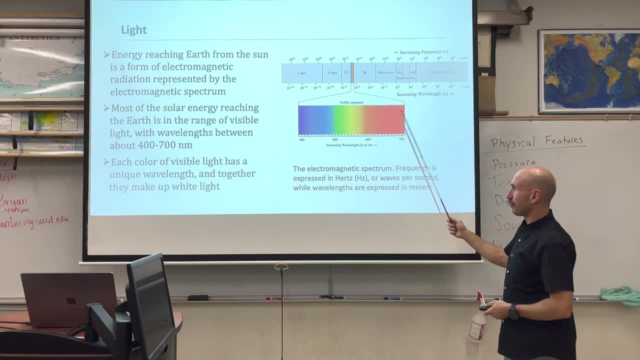 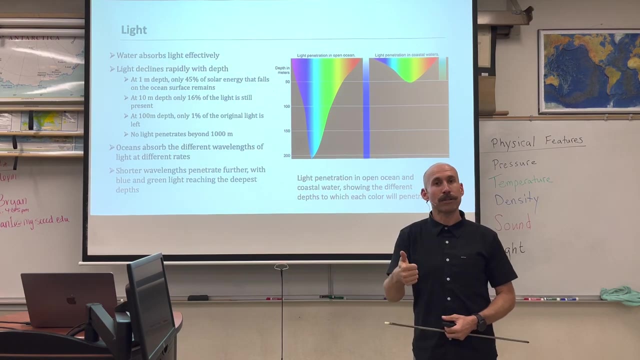 in their varying wavelengths. We bring all of the slide together, We have white light or which is its own unique wavelength. Okay, so light in the ocean. We've talked about the photo zone, dysphotic zone and aphotic zone. actually, 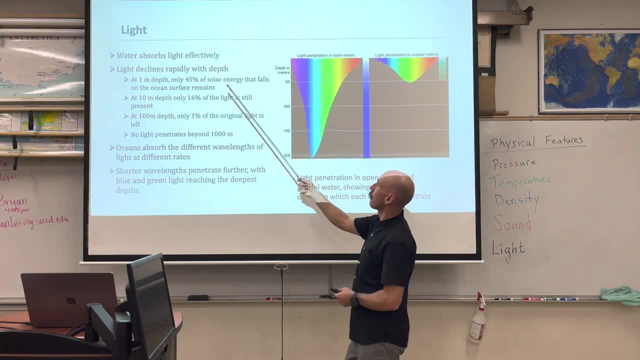 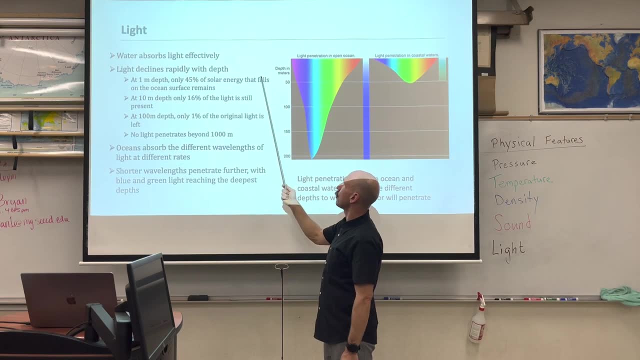 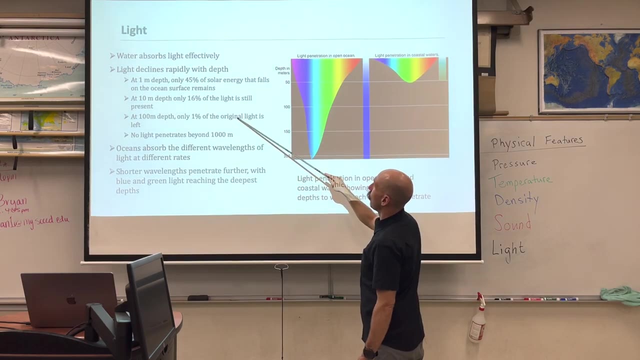 That's probably on the next slide, but at one meter we get to the first layer. yeah, about this. tall, about three feet, about a yard or so. uh, only 45 percent of the solar energy that hits the ocean surface remains at 10 meters, 16. at 100 meters, one percent, and then so much less. 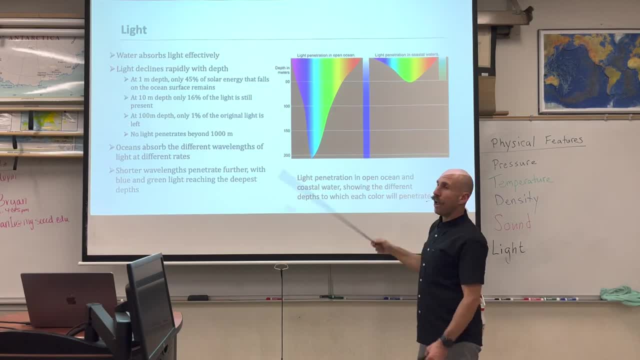 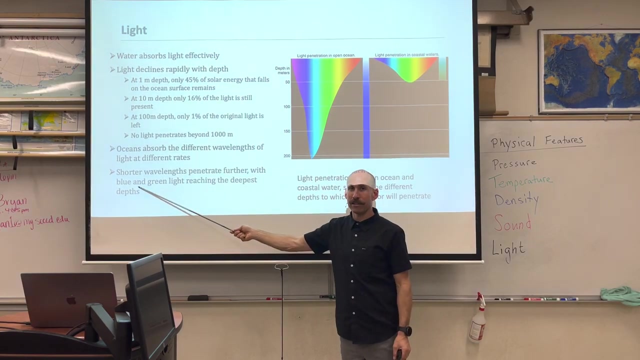 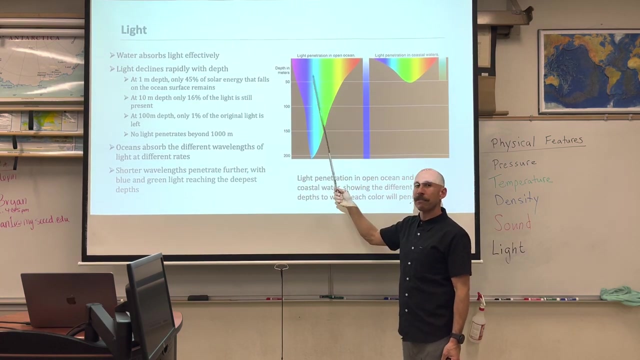 when you get down to a thousand meters. now, where's all this light going? well, it's being absorbed. the ocean absorbs different wavelengths of light at different rates. the shorter wavelengths penetrate further, with the shortest wavelength penetrating the furthest being the blue lights. so why are oceans blue? because all the other colors in the electromagnetic spectrum are absorbed. 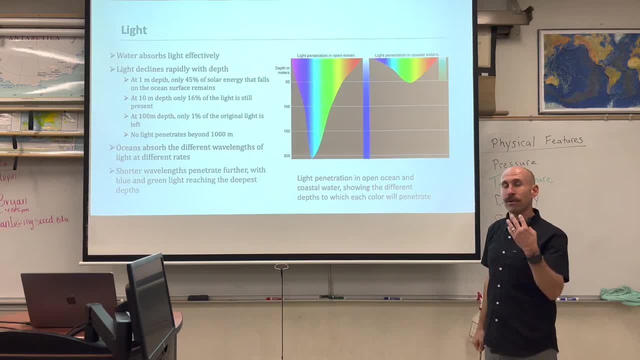 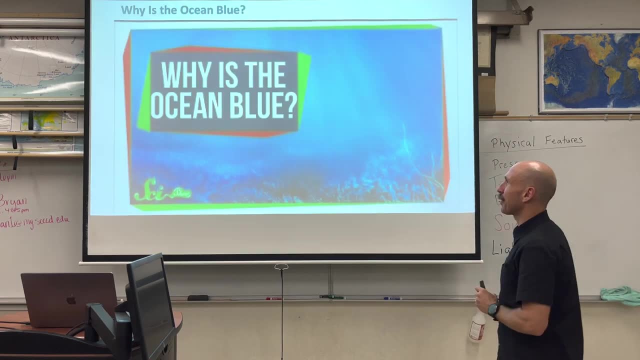 leaving the only thing left, which is blue, and that is what we see. also green. sometimes ocean water is blue and that is what we see. look green, the nuances of ocean. it makes them really cool. so check out the video. why is the ocean blue? it will summarize what i just said quite nicely. 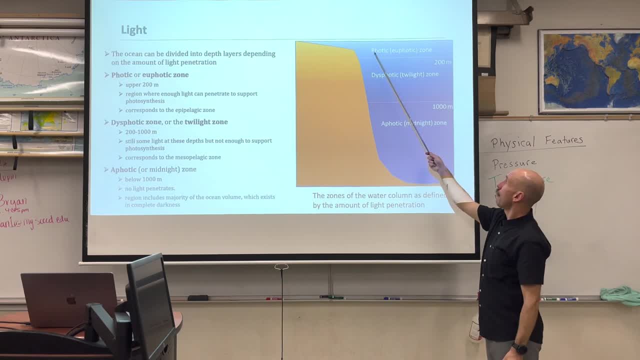 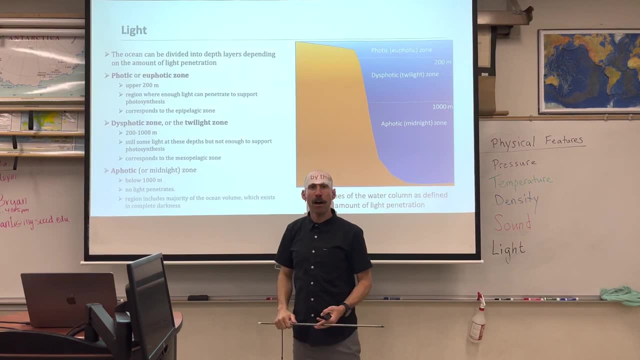 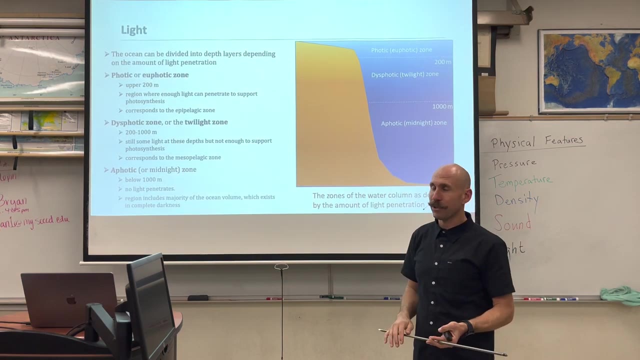 here is the slide: photic, dysphotic and aphotic. so we have a zonation of the ocean environment by depth with. i know we love to classify things. it's what scientists do: we label, we identify, we organize and we classify. and as far as light goes, there's the photic, the 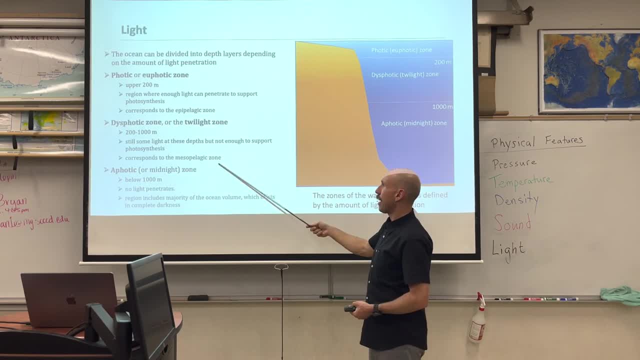 upper 200, the dysphotic 2 to 100 and the aphotic below a thousand meters. no light penetrates, complete darkness and really amazing adaptations for marine life that exists in this area. uh, upper 200 meters, this is where the action is happening. this is the mixed layer for temperature. this is 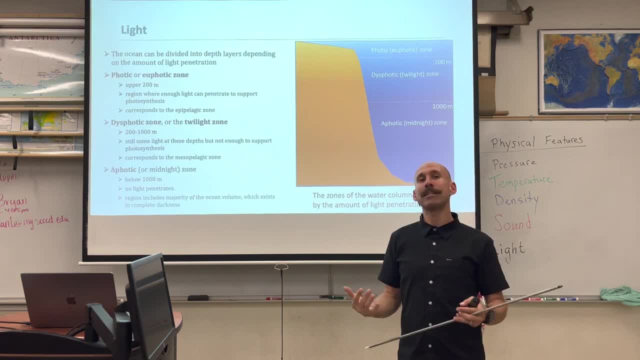 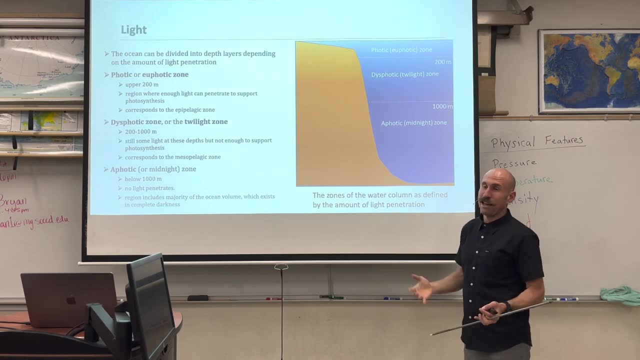 where photosynthesis is occurring. this is where abundant amounts of marine life are living, and it makes sense because light is one of the primary sources of energy for all life on earth, except deep in the oceans. at hydrothermal vents we have the process of chemo chemosynthesis, where entire communities survive off of the bacteria that produce energy from the